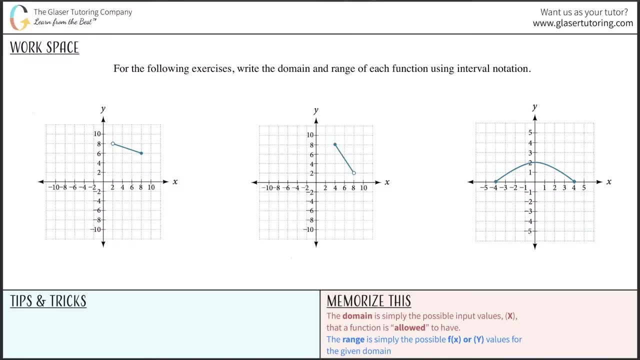 For the following exercises: write the domain and range of each function using interval notation. All right, so remember down here, guys. we just want to remember these couple of facts. The domain is basically the set of x values that you're allowed to have. 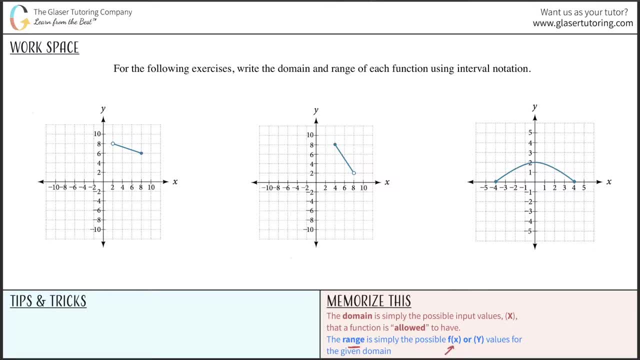 and the range here is simply the possible f of x aka y values that can be obtained given the domain. All right, so x is domain, basically, and y is range. So if I were to look at the first graph, I notice I want to think about the span of x values. So I notice that we have an open circle. 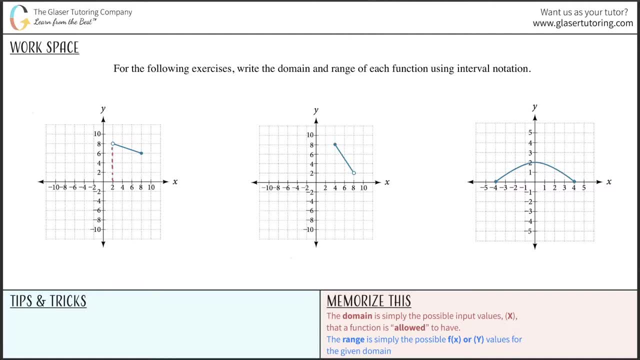 here, at x is equal to 2.. We also notice that we have a filled-in circle. at x is equal to 8, and the graph says that we can have any value in between. All right, the x is 2 and x is 8.. 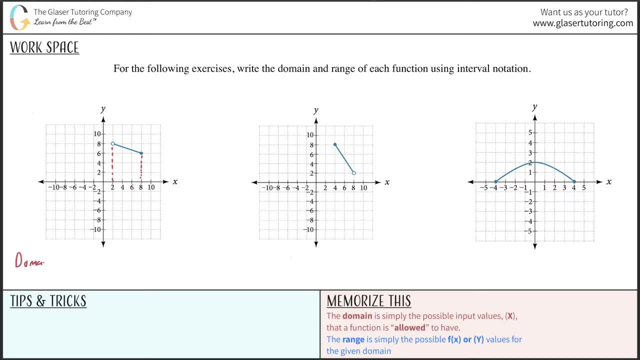 So now keep in mind, for the domain. here, for the domain, using interval notation, we cannot include, because it's an open circle, 2. So therefore it's going to be 2, exclusive. That's the purpose of the parentheses Comma, then inclusive, all the way to 8, okay and inclusive. 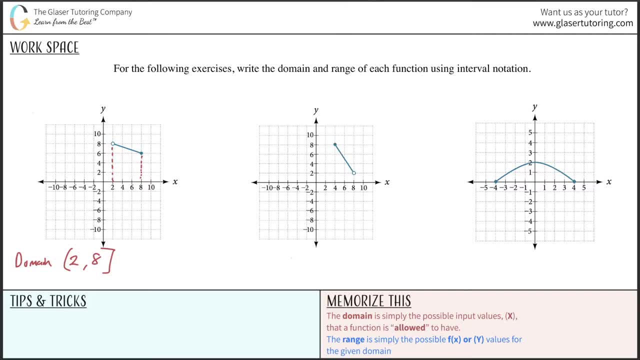 of 8.. So that is denoted with the bracket. So this would be the domain for this graph And the function now is just the set of x values. All right, so now let's look at the set of y values. okay, So if you notice, the graph goes out to: a has a y value of 6 when x is. 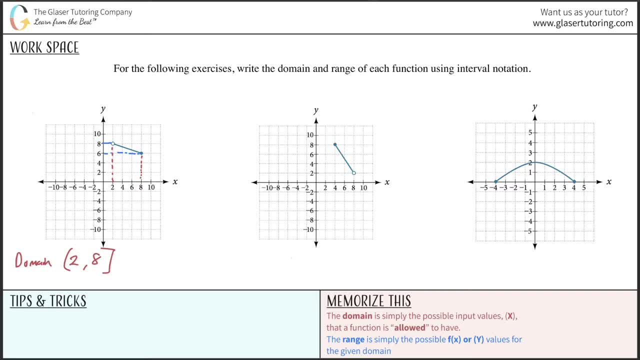 8, and it goes up to a point of 8, but it doesn't equal 8 because it's an open circle. So, similarly, when we think about range, so when we think about range, we're going to have the values of going. 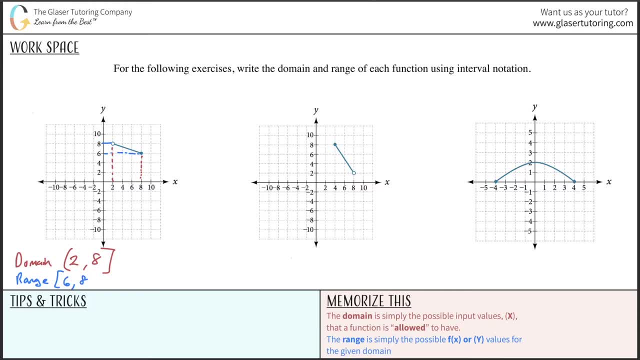 from inclusive of 6 all the way to 8 exclusive. All right, apply the same logic to this one. So we realize it goes from x is 4 to x is 8, but not including 8.. So therefore the domain here.